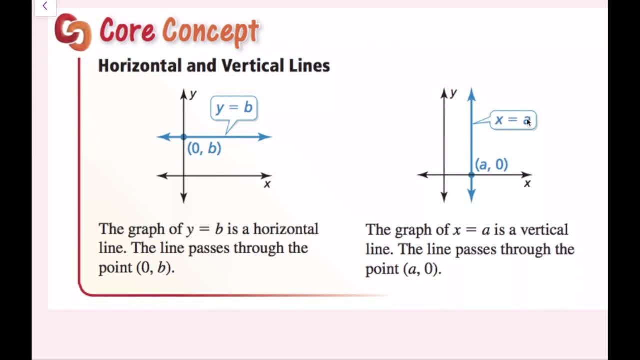 opposite situation: x is going to equal our constant a value, and it doesn't matter what my y value is, because x is always going to be that a value and this is a vertical line. Just a reminder: this is a function. this is not a function. 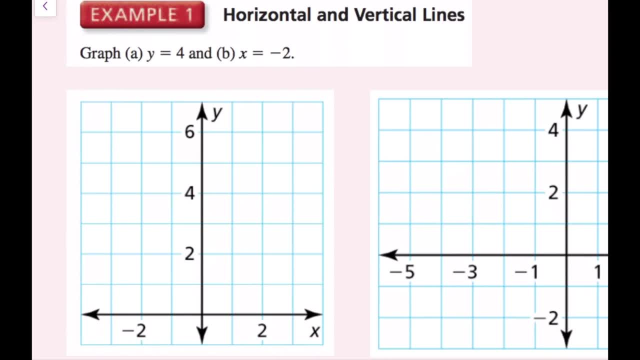 So we're going to graph y equals four. and then we're going to: graph x equals negative two. So to graph y equals four. you could always make a table of values, you can always do that, and vertical lines. you can just recognize that, since I have, y is equal to a constant. 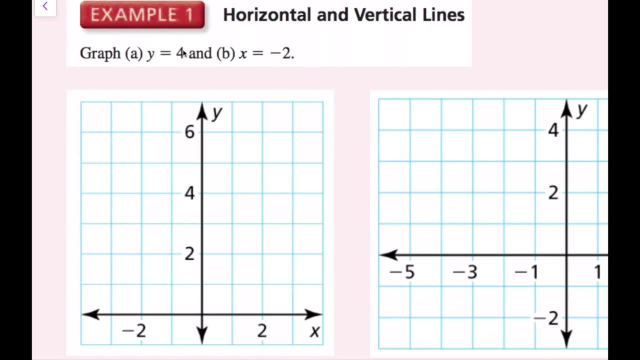 I'm just going to have a horizontal line at the y value of 4.. So this is my 4y value and all of my x values are going to be y. So if I wanted to draw points, I could, I could draw a. 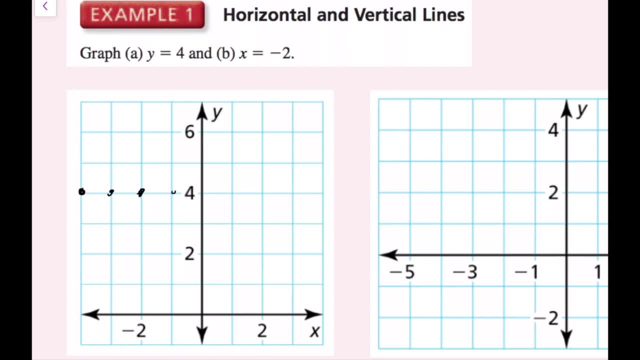 point right here, here, here, here and so on. I could draw as many points as I wanted to, because I know that y is going to be equal to 4, regardless of the x value. And now I'll take my straight edge. 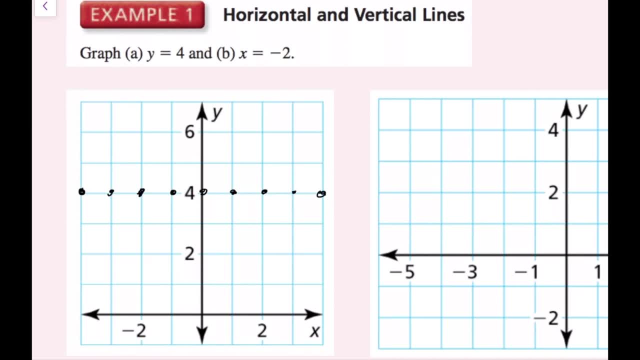 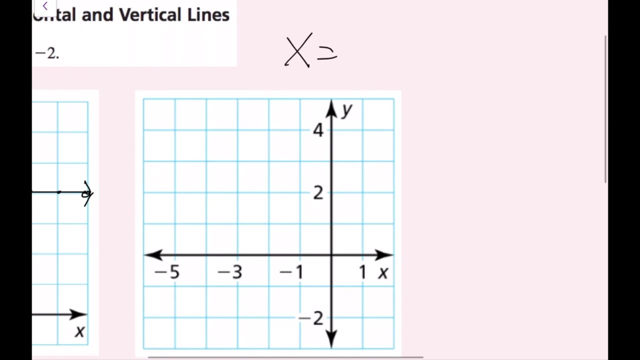 and draw a line through all of my points And then put arrows on your line to show that it is infinitely long. And now we're done with the first part. For the second part, I'm going to: graph x equals negative 2.. I'm just going to write that down. And same thing In this case. 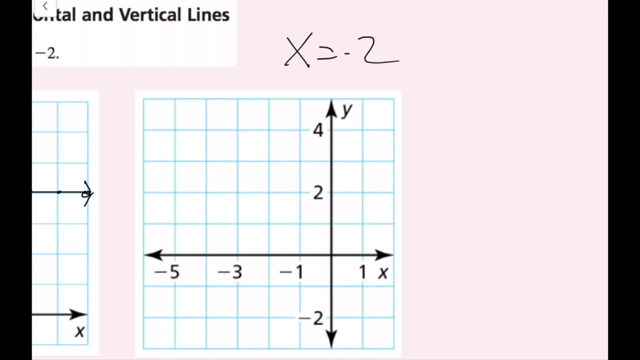 we're going to have a vertical line, because I have an x value by itself, with a constant, And all my x values are going to be equal to 4.. So I'm going to draw a line to negative 2.. It doesn't matter what y is, So I find negative 2. 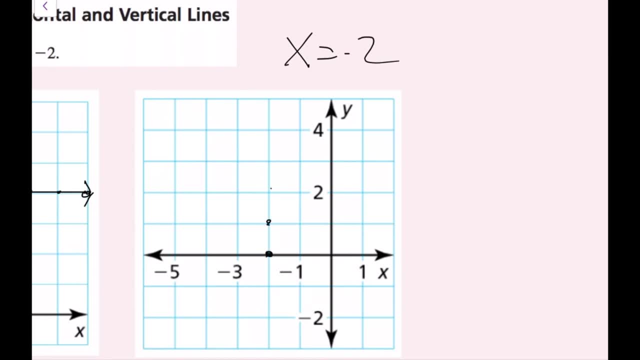 right here, And it doesn't matter what my y value is, because I know that the only piece of information is that x is negative 2.. So I'm going to draw my points. You don't have to do this. by the way, You don't have to draw all your points. I'm just doing this to show you that. 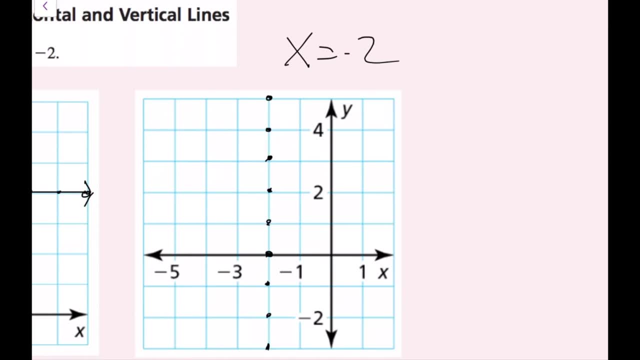 every x value is negative 2 here. So I'm going to draw my points like I did. I would just recommend drawing, if you're going to graph this, doing the top point and the bottom point, because the farther away your points, the more accurate your line will be when you graph it. 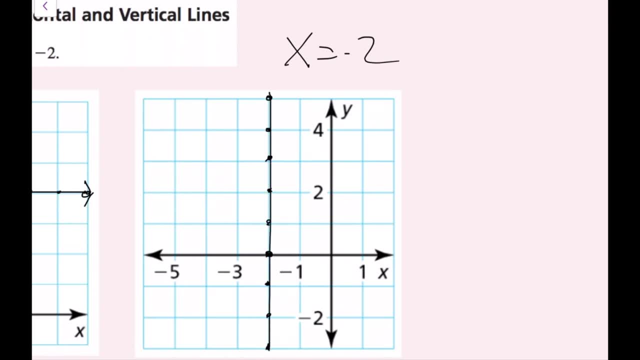 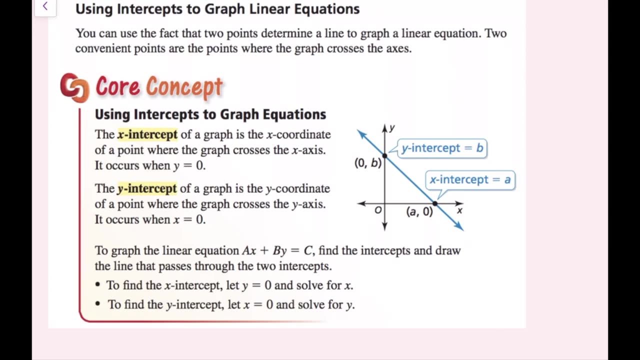 And then, once again, take your straight edge, draw your line through and then include your arrows, And then we're done with this one. So now we're going to use intercepts to graph linear equations. You can use the fact that two points determine the line to graph a linear 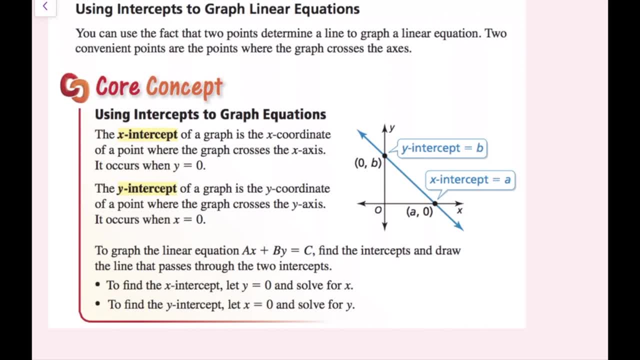 equation. Two convenient points are the points where the graph crosses the axes. The x-intercept of a graph is the x-coordinate of a point where the graph crosses the x-axis. It occurs when y equals 0.. An easier way to think of that is: the x-intercept is the value of x. 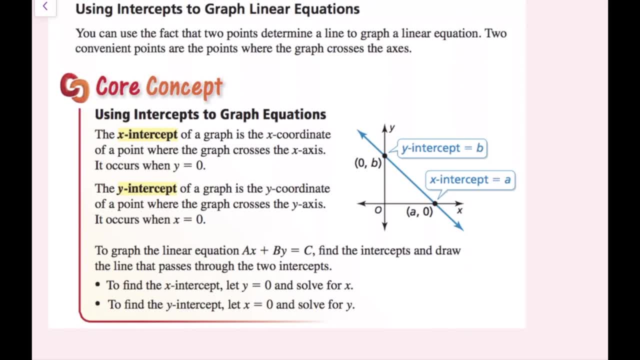 when y equals 0.. The y-intercept of a graph is the y-coordinate of a point where the graph crosses the y-axis. It occurs when x equals 0.. Another way to think of that is: the y-intercept is the y-value when x equals 0.. To graph the linear equation ax plus by equals c, find the intercepts. 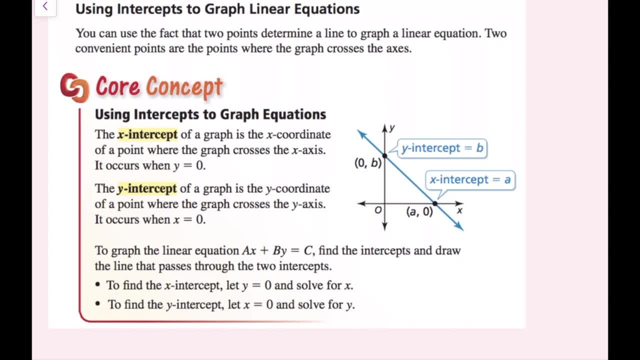 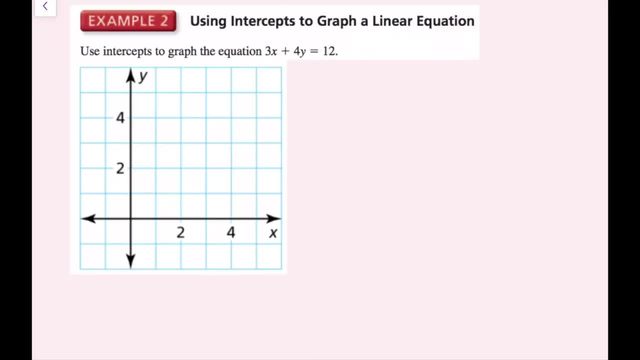 and draw a line that passes through the two intercepts. To find the x-intercept, let y equals x. To find the y-intercept, let x equals 0 and solve for y. So for this example, we're going to graph this equation: 3x plus 4y equals 12, using our 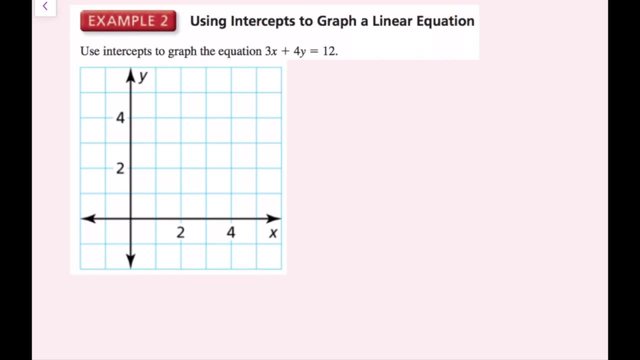 intercepts. So first I'm going to find the x-intercept. So to find the x-intercept, remember the x-intercept is the value of x when y equals 0. So all I'm going to do is plug in 0 for y. 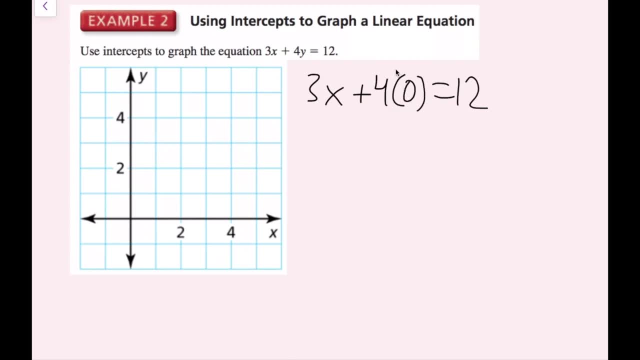 I'm going to rewrite this down. This can just get into the habit of getting rid of that term. I'm going to rewrite this as just 3x equals 12.. Now just solve for x. so divide 3 on both sides, I get x is equal to 4.. So my x-intercept is 4.. The point that corresponds with this: 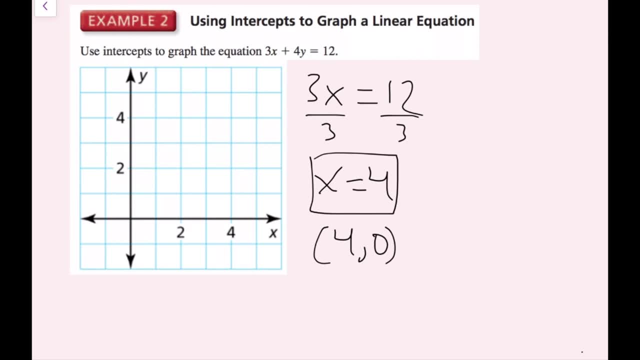 is Because, remember, the x-intercept is the value of x when y equals 0.. So when x equals 4y equals 0, okay. So I'm going to graph this point: 4, 0.. It's right here on the x-axis. 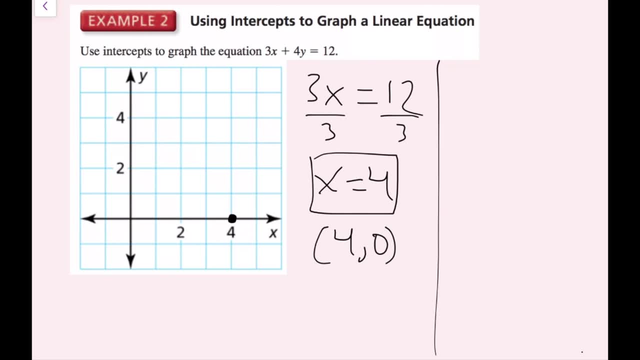 Now I'm going to do the same thing, but find the y-intercept. Remember, the y-intercept is the value of y when x equals 0. So I'm going to plug in 0 for 3x, But if you remember, this whole entire 3x term is just going to go away. 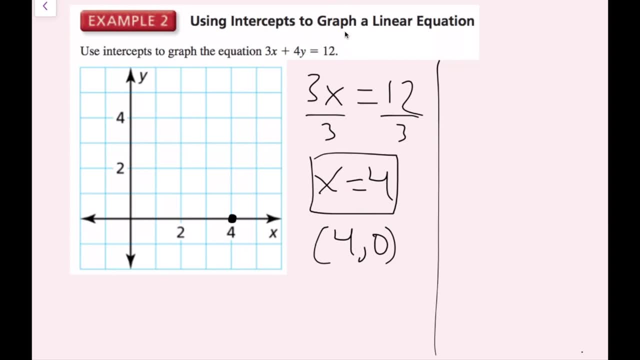 So I'm just going to get 4y equals 12.. I'll divide 4 on both sides. I'll get y is equal to 3.. And remember, the y-intercept is the value of y when x equals 0.. 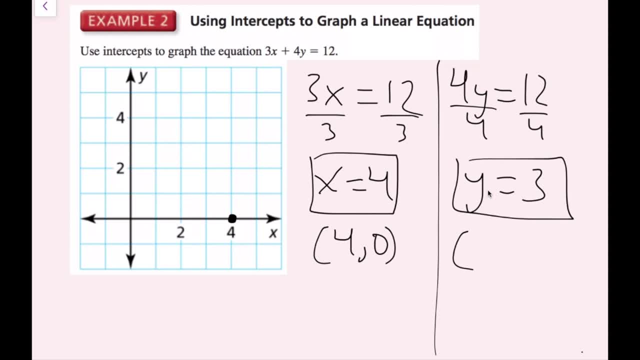 So y is 3 and x is 0.. So my ordered pair is going to be 0, 3.. And that is right here on the graph. The last step is to just draw a line through these points using my straight edge. 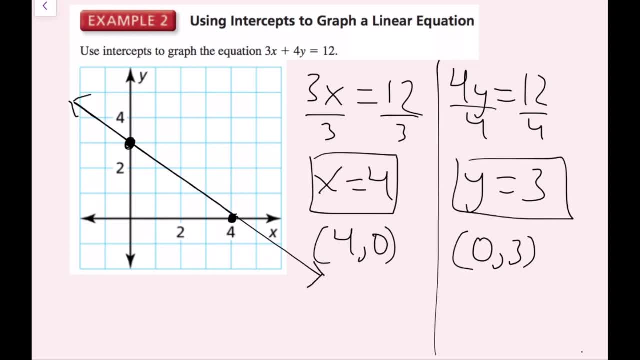 And draw your arrows, And I recommend having your Line extend on the entire graph. If anything, have it go off a little bit. It's a little bit harder for me because I'm using a stylus and an iPad, But on paper it's much easier to graph. 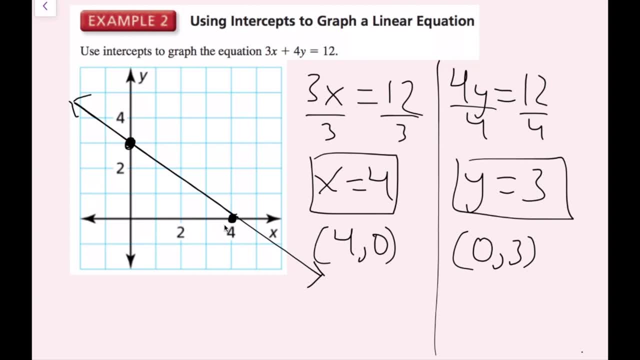 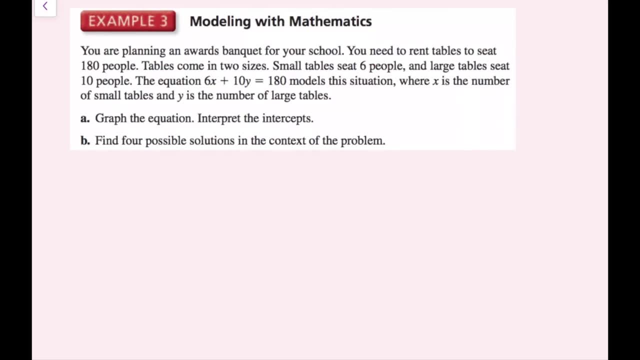 Anyway, we've successfully drawn our line through our two intercepts And now we're done with this one. You are planning an awards banquet for your school. You need to rent tables to seat 180 people. Tables come in two sizes: Small tables seat 6 people and large tables seat 10 people. 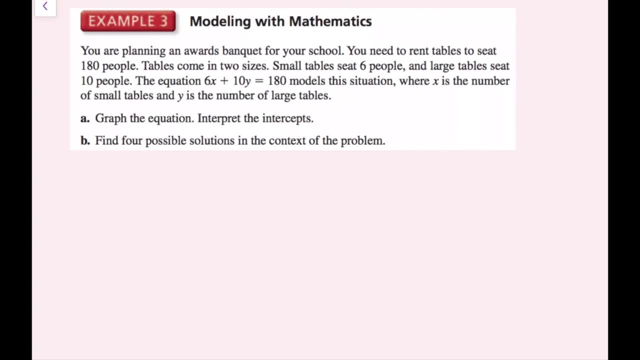 The equation: 6x plus 10y equals 180. models this situation where x is the number of small tables and y is the number of large tables For part a, graph the equation, interpret the intercepts. So we're going to graph this equation by finding the x-intercept and finding the y-intercept. 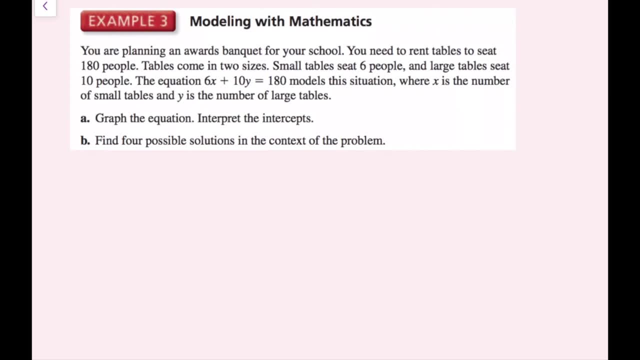 and then plotting those two points and then drawing a line through those two points, So to find the x-intercept. it's when y equals 0. So I'll do 6x And then if I plug in 0 for y, that whole term goes away. 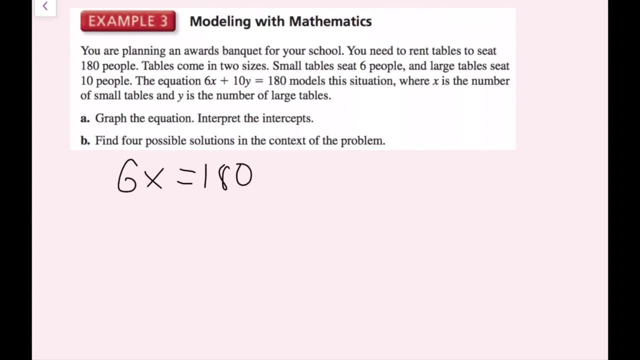 So this 6x is just equal to 180.. I'll divide 6 on both sides and then I get x equals 30,, okay, So the point that corresponds with this- x equals 30, is 30 comma 0. 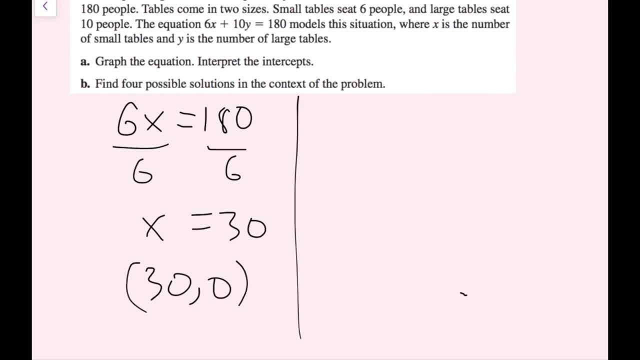 So this is one of the points I'm going to plot For my y-intercept. I'll plug in 0 for x, So this whole entire 6x term goes away. So I just have: 10y is equal to 180.. 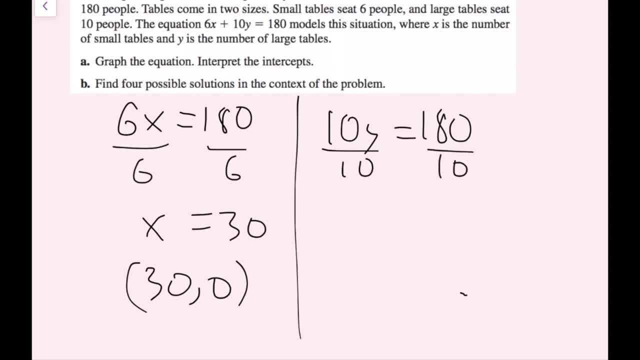 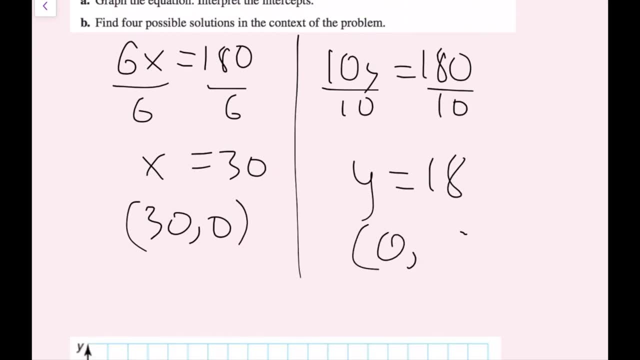 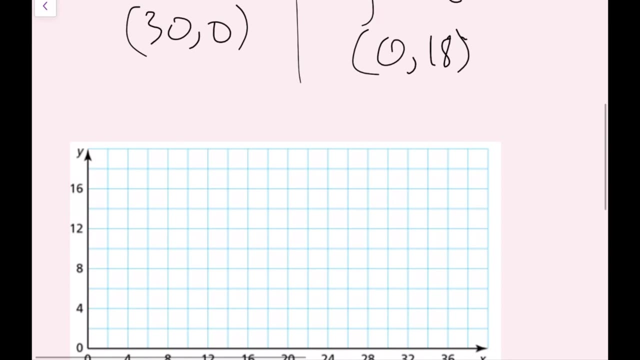 Divide 10 on both sides, or you could just cross out a 0 on both sides- You get y equals 18. And the corresponding ordered pair for that one is going to be 0 comma 18.. So now all I have to do is plot these points and then draw a line through it. 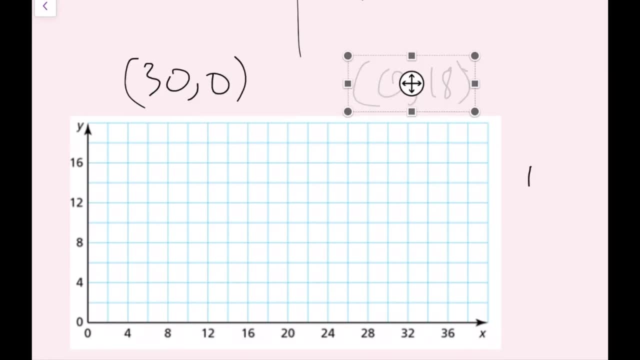 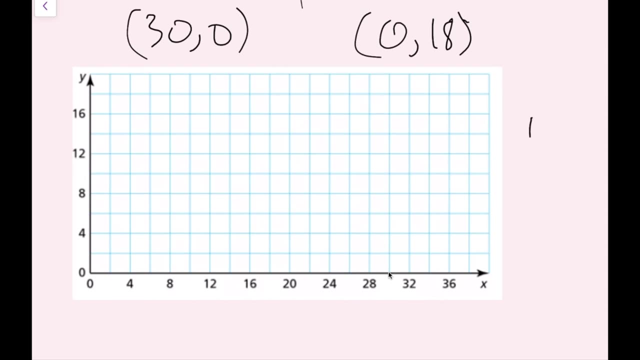 So I'm going to actually bring these points down. So on my graph I see the point 30 comma 0 is right here where my mouse is, So I'm going to put that right there. And then my other point is going to be 0 comma 18, which will go right here. 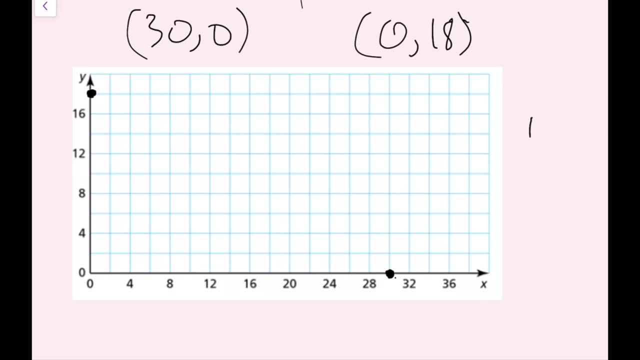 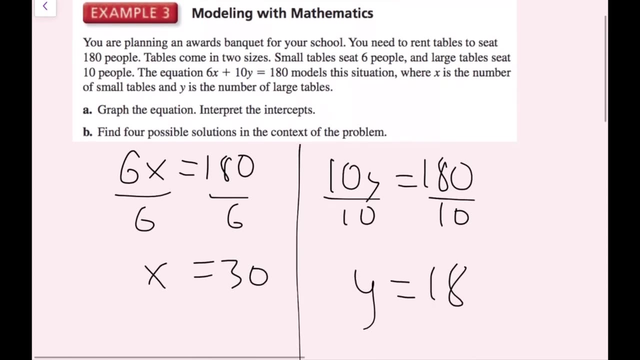 And now I want to actually not draw a line through this, but just a line segment, Because if you look at the context of the problem, scroll back up here: x is the number of small tables and y is the number of large tables. 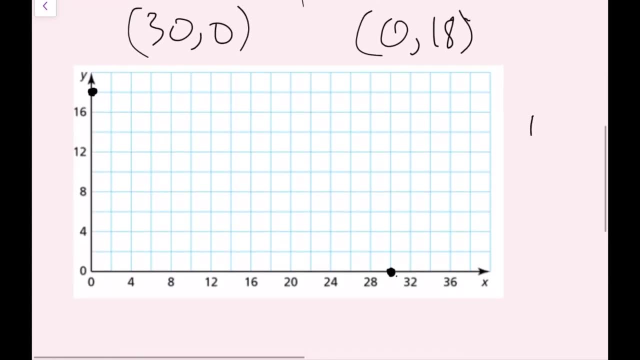 It doesn't make sense to have a negative amount of small tables or a negative amount of large tables, So we're just going to be sticking with quadrant 1 here. Anyway, I'm going to align my straight edge And I drew as best of a line as I could with my stylus. 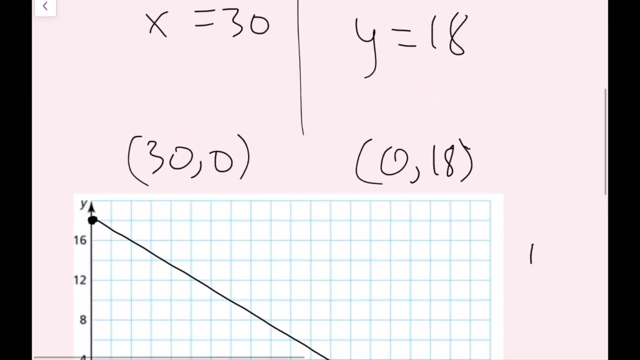 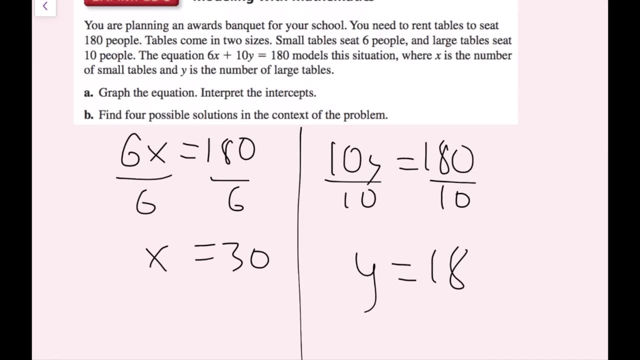 So we're done with part A, So I'm going to scroll back up. Part B says to find four possible solutions in this table. So I'm going to find four possible solutions in the context of the problem Now, because my graph is hand-drawn on my iPad using my stylus and a flimsy straight edge. 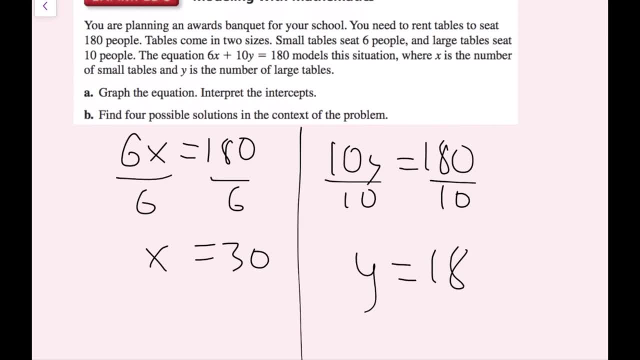 my graph is not going to be as accurate as possible. Your graph on paper will be much more accurate. But for this part- part B- I'm going to go to Desmos, which is an online graphing calculator, And I have this exact function graphed. 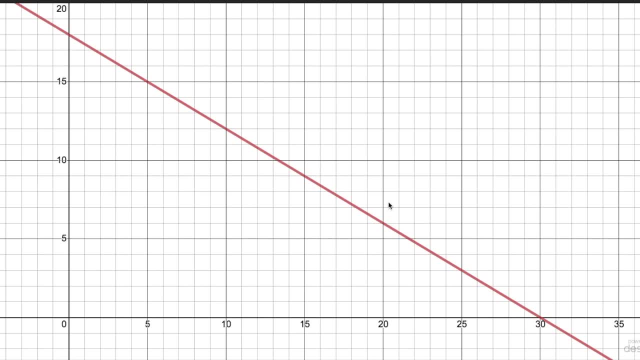 So this is the same line, except for this time it's going to be more exact. So we need to find four possible solutions in the context of the problem. Well, if we remember, x is the number of small tables and y is the number of large tables. 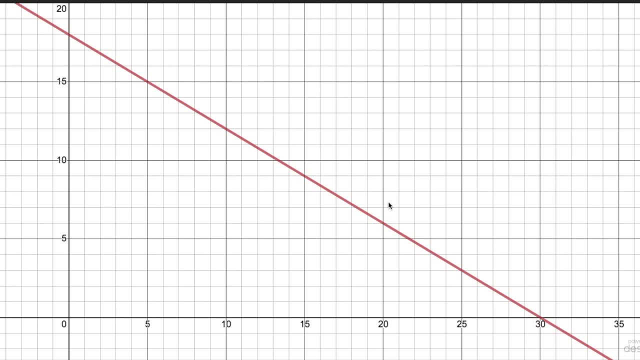 So I am not going to be able to have like 2.785 or some sort of fractional number of tables, So really I should have a discrete domain here. So I really just want to find some whole number solutions. Well, right here, the intercept is 30, 0..